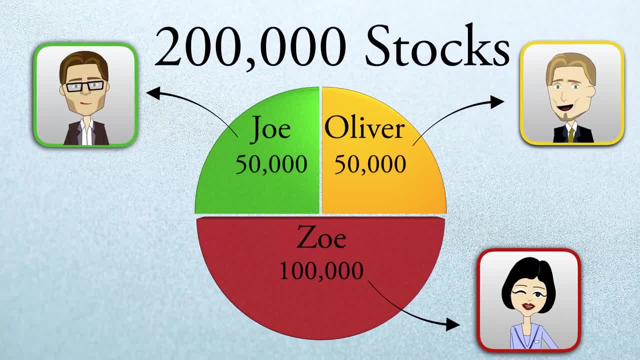 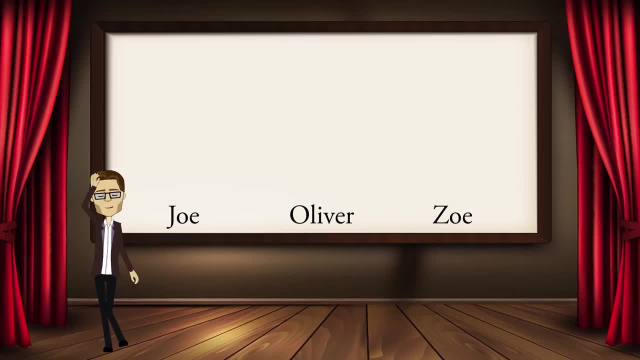 but the shares that grew to 200,000. shares Outstanding, What does the ownership and control of the company look like now? Joe controls 50,000 of 200,000, equals 25%. Oliver controls a similar stake: equals 25%. Zoe controls 100,000 of. 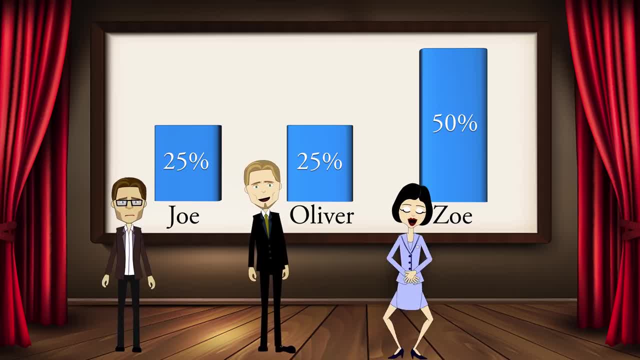 200,000, equals 50% of the company. Joe's and Oliver's relative part in the company just shrank. And with respect to control, now just Zoe, with 50,000 shares Outstanding controls 100,000 of 20,000.. 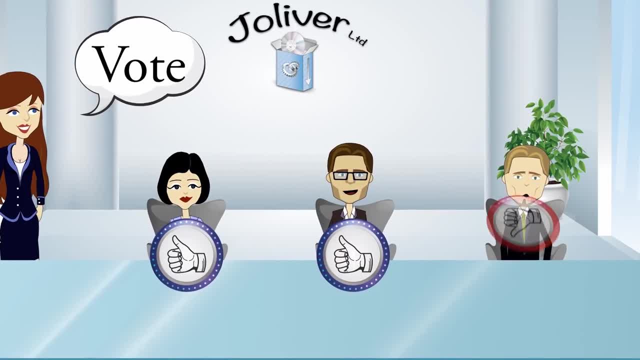 Joe controls 50,000 of 200,000, equals 25%. Oliver controls a similar stake equals 25%. Zoe controls one of the shareholders. support could decide what the company does when 51% majority is needed, even if the other original owner disagrees and votes. 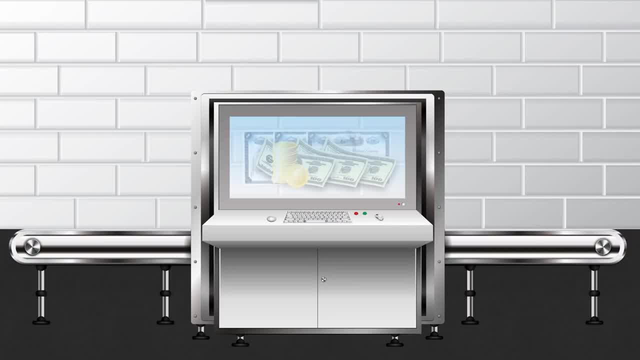 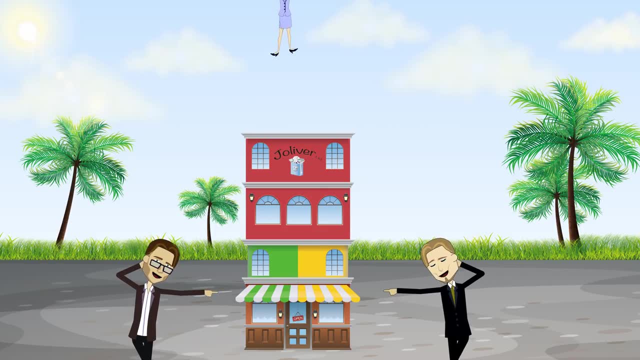 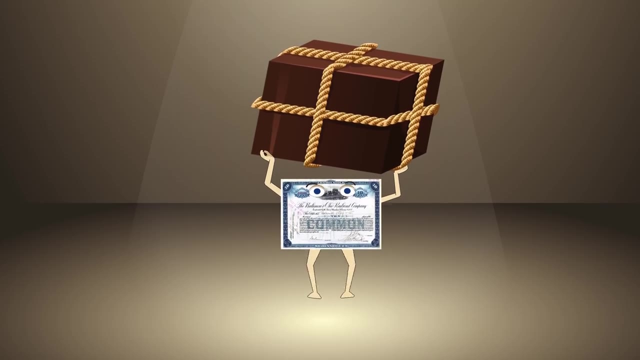 against the proposal. this phenomenon- the printing of stock by the company which reduces the relative size of the asset held by existing shareholders- Joe and Oliver in our case- is called dilution. it dilutes, takes away the potency and power of each and every pre-existing stock. printing more shares means nothing for 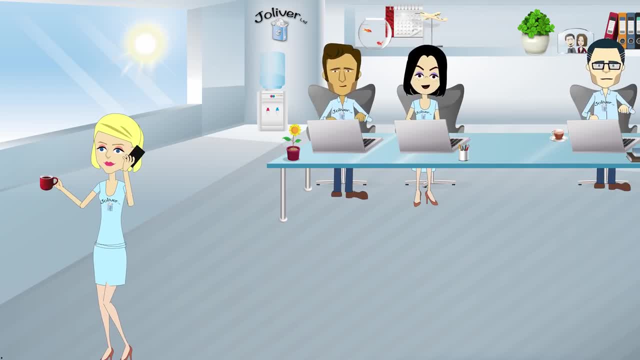 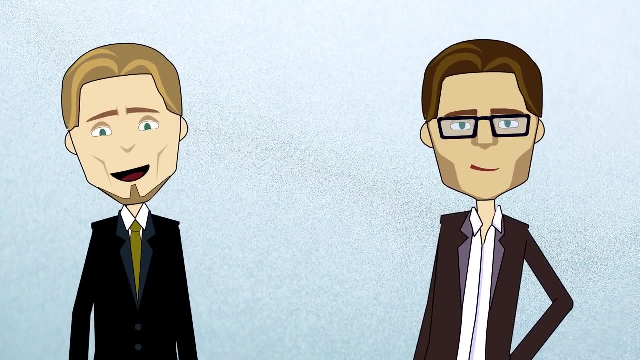 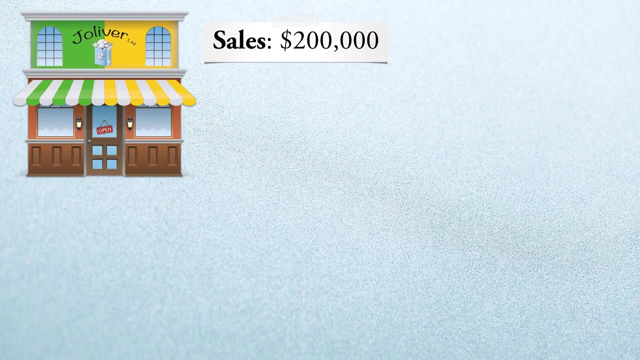 the clients and managers of the jaw loved her limited. it's still the same company delivering the same products or services. it is another thing altogether for the shareholders, of course. let's imagine that prior to purchasing Danny's codes, limited jaw, Oliver limited, sold software for $200,000 per year and earned 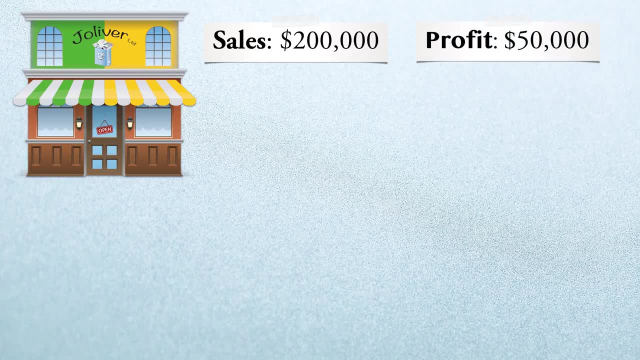 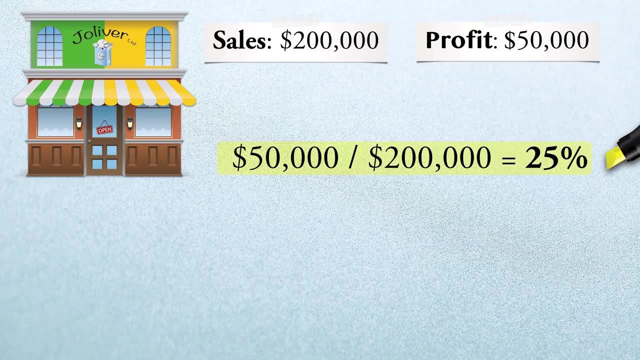 $50,000 in profits per annum before tax. that is not bad. fifty thousand dollars of $200,000 equals twenty-six hundred thousand dollars in profits per annum before taxes. before tax, 25% return per annum on their capital investment. Let's pretend Danny's Codes Limited brought in an additional $200,000 per year in earns. under Jolliver employees and cost basis, an additional $60,000 in profits. That's even better since $60,000 of $200,000 equals 30% annual return on the new capital. The new business is $400,000 per annum and the business nets $110,000 in profits per. 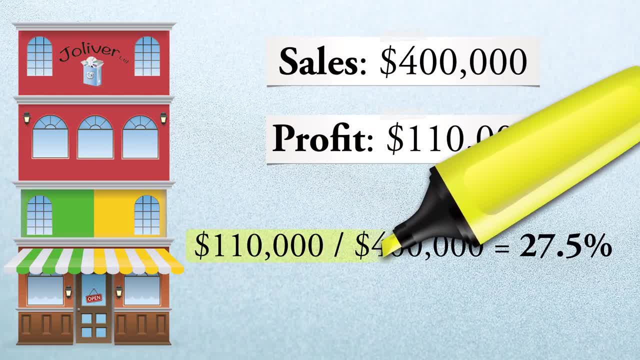 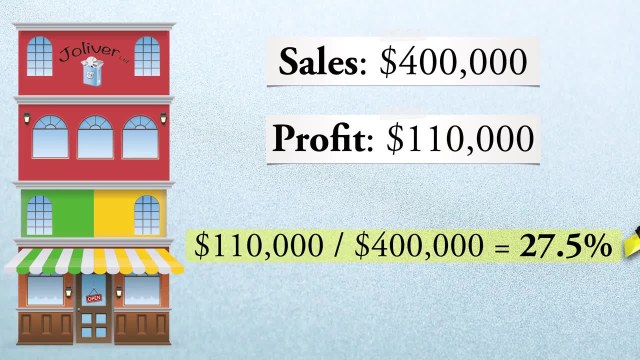 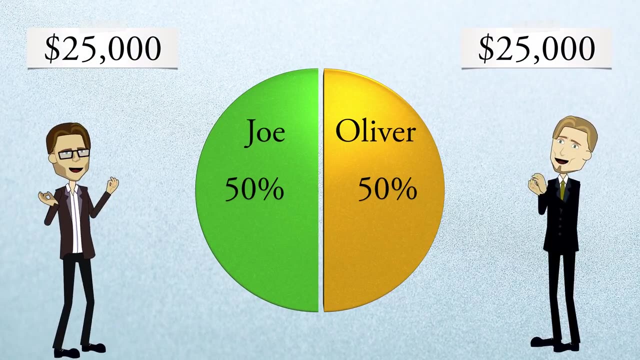 annum, which is 27.5% return on capital business, an improvement from the older 25%. The new Jolliver Limited is not only a larger firm that is stronger, but it is also more profitable. Before the dilution, Oliver and Joe each controlled $25,000 worth of profits. 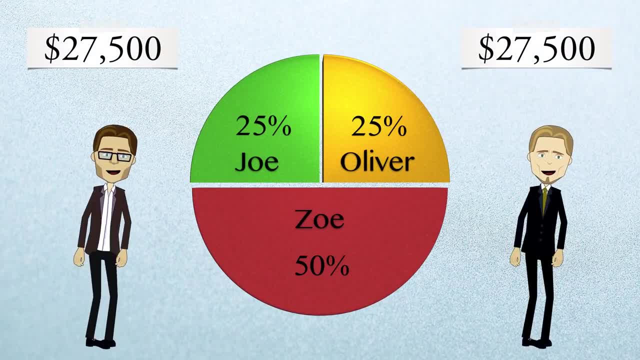 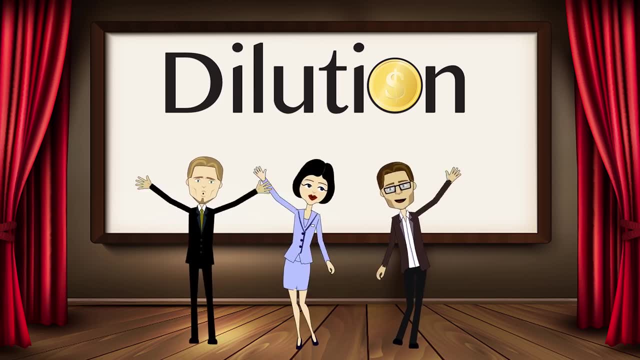 Today, after the dilution, they each control $27,500 worth of profits. In essence, they own a smaller slice of a bigger and better cake. It is an unfortunate fact. It is also an unfortunate observation that managers are much more likely to mess up the